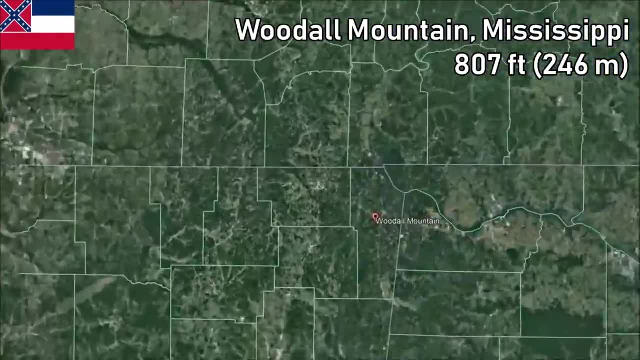 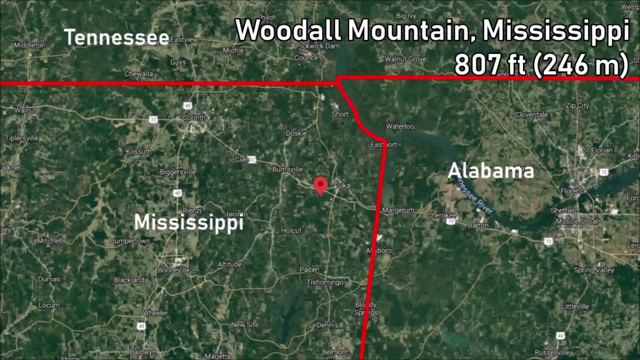 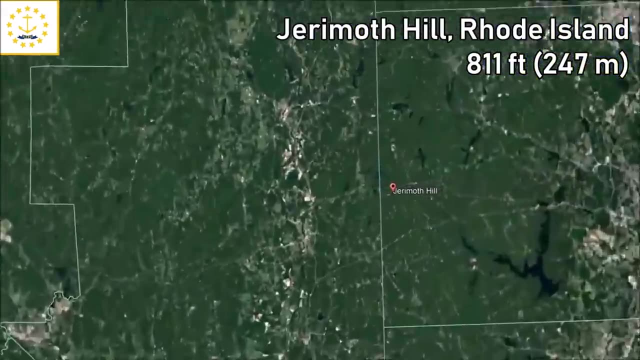 Neighboring Mississippi has a similar high point, Woodle Mountain, with an elevation of 807 feet. Again, it's just one hill of many found in the very far northeast corner of the state, near the Tennessee River. Returning to the Atlantic coast, Rhode Island has Jerimoth Hill, an 811-foot hill about a mile from the border with Connecticut. 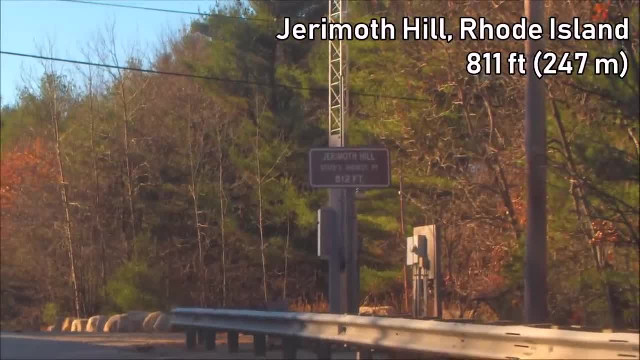 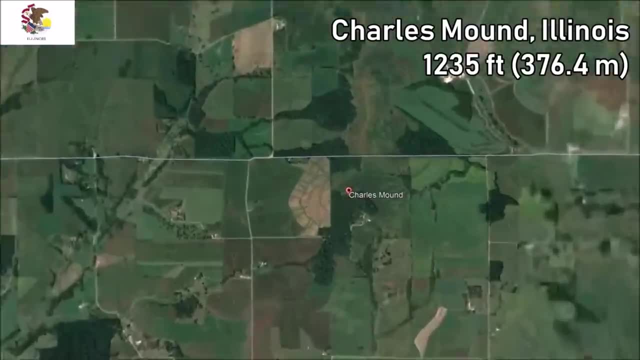 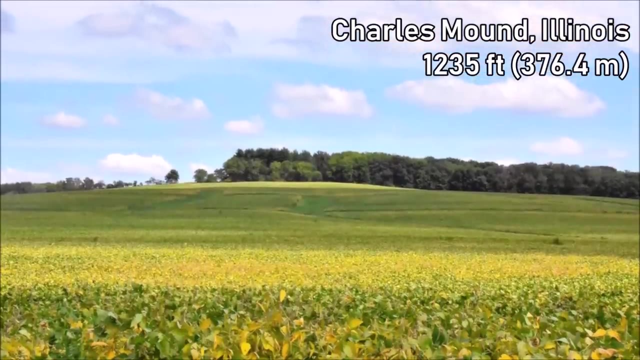 Not much to see here, once again, as it's barely noticeable in the surroundings. The first inland state to make the list is my home state, Illinois. Despite being notoriously flat, Illinois does have some hills in the northwest and southeast. Charles Mound, the highest of these is the first high point on the list, with over 1,000 feet in elevation. 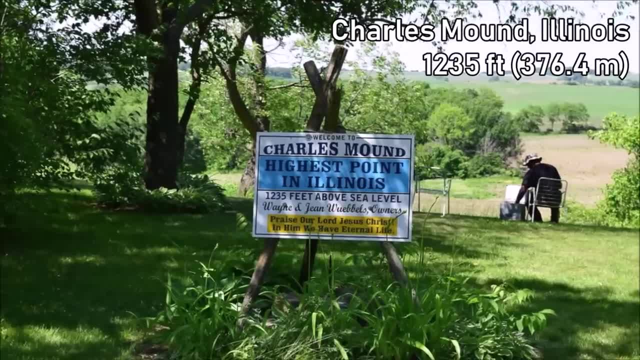 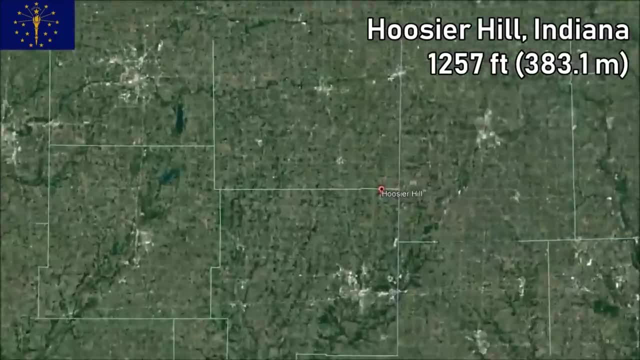 At 1,235 feet. Charles Mound is on private farmland bordering Wisconsin in the far northwest part of the state. Next-door neighbor, Indiana, has a very similar high point, Hoosier Hill, just a couple miles from the Ohio border. 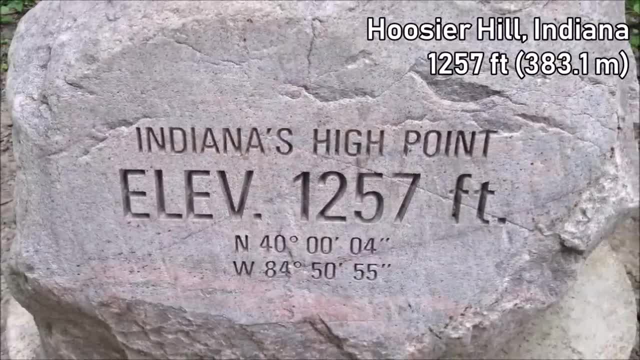 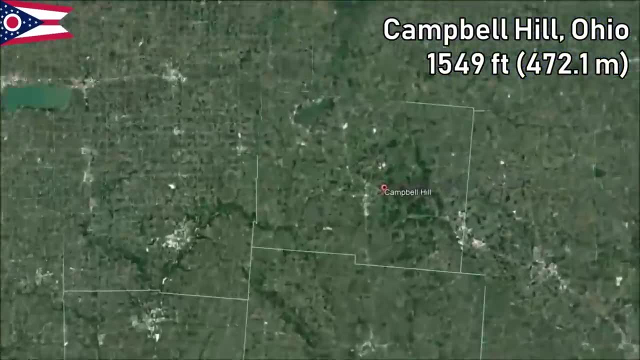 It too is on private property and it also has a very similar elevation to Charles Mound at 1,257 feet. We head one way to the north and then to the south. We head one state over again to Ohio and its highest point, Campbell Hill. 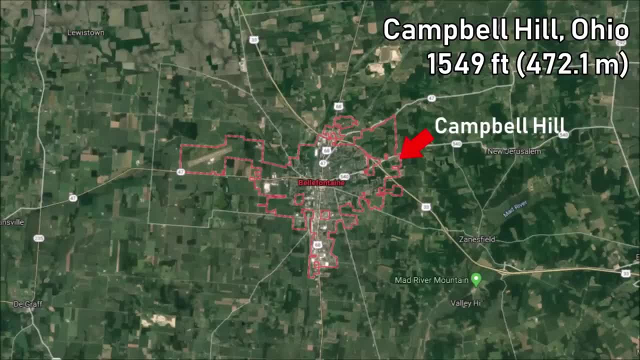 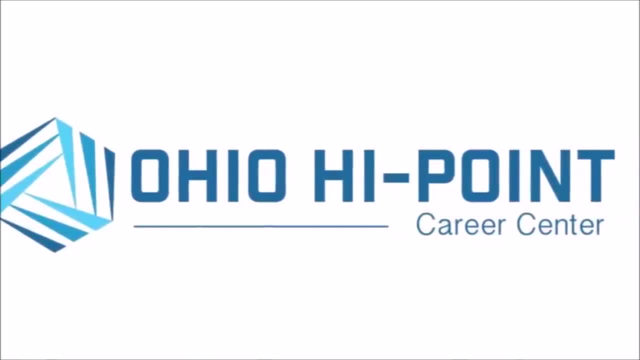 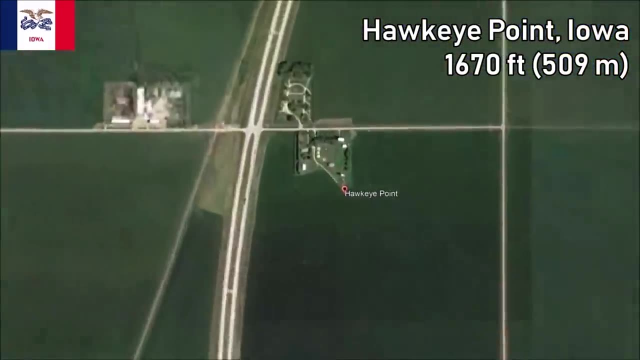 This one is found in the town of Bellefontaine, with an elevation of 1,549 feet, and is home to the aptly named Ohio High Point Career Center, which is a technical school for adults. Continuing this string of Midwestern states is Iowa, which is home to Hawkeye Point. 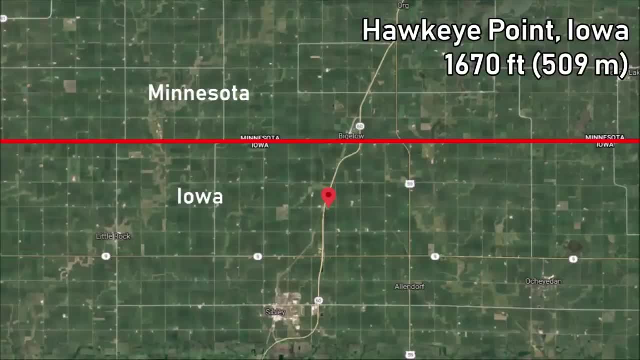 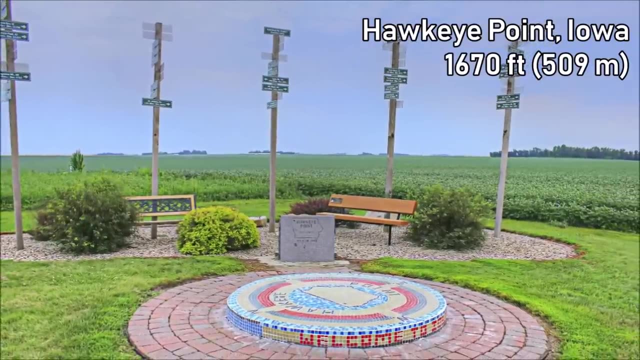 At 1,670 feet. it's a couple miles from the Minnesota border in the northwest of the state, with a very cool mosaic and signs pointing to the other 49 state high points. Missouri brings us the first high point that is actually a mountain of sorts: Tom Sock Mountain. 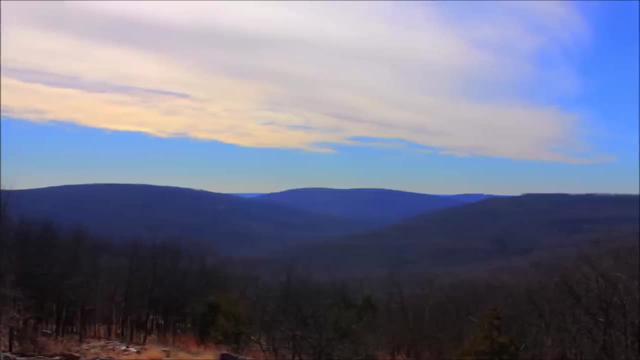 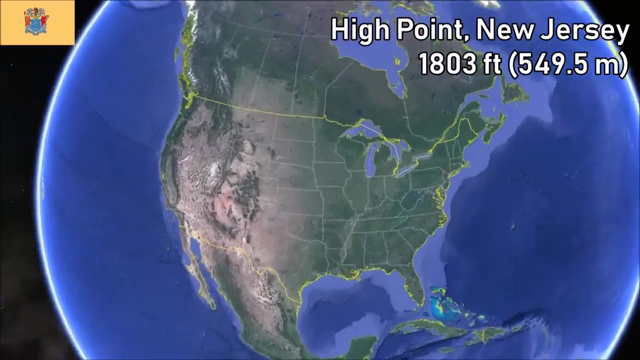 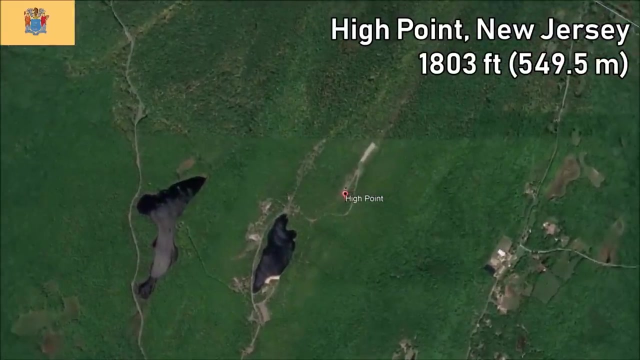 At 1,772 feet. it's not that tall, but it is found in the St Francis Mountains of the Mark Twain National Forest. We return once again to the coast with New Jersey's high point, named High Point. Great job, New Jersey, always bringing that innovation to the table. At 1,803 feet. High Point is found within High Point State Park in the far northwestern corner of the state. It's the most grandiose of the high points we've seen so far, as it features a 220-foot-tall obelisk on its top. It's back to the Midwest with my friendly neighbors to the north Wisconsin. Their high point, Timms Hill, is at 1,951 feet in elevation and is found in the hilly wilderness of northern Wisconsin. It has an observation tower at the top of it. 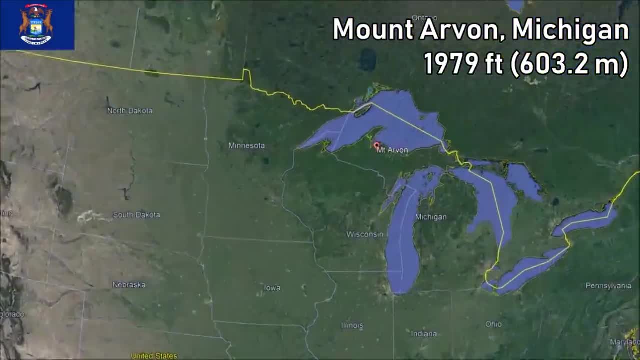 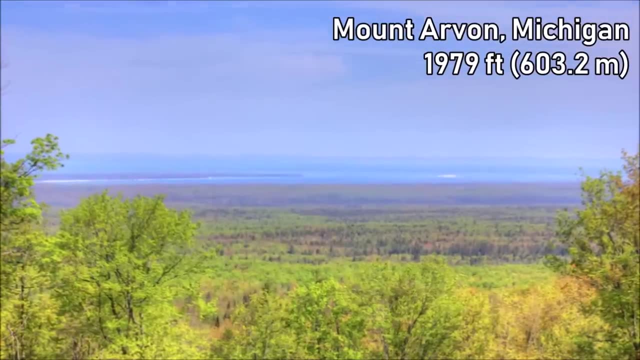 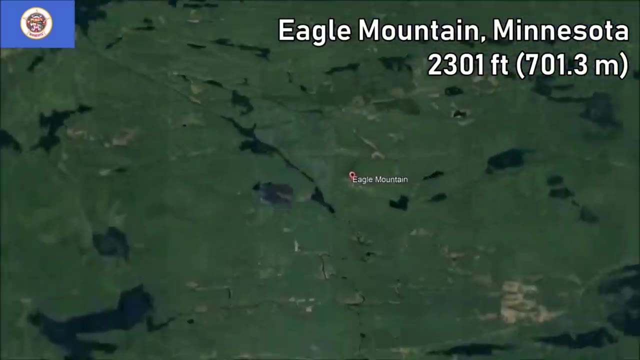 Heading even further north to the UP, Michigan's highest point is not too dissimilar to Wisconsin's. Mount Arvin is at an elevation of 1,979 feet and is part of the Huron Mountains Across Lake Superior. in the far northeastern tip of Minnesota is Eagle Mountain, with an elevation of 2,301 feet. 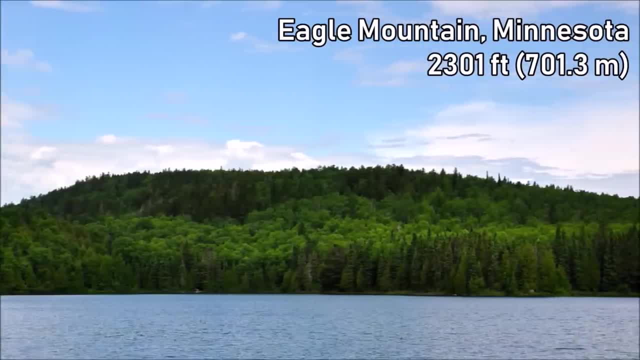 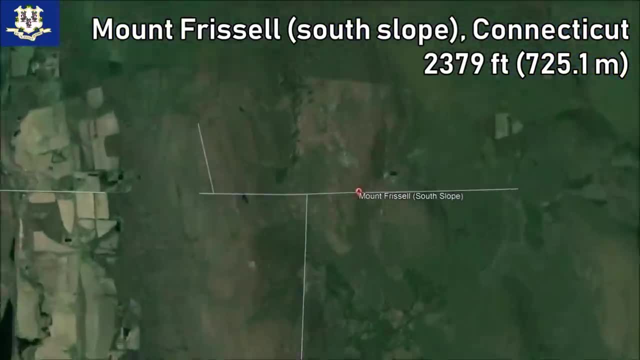 It's set among the rugged and beautiful hills of the Superior National Forest. Connecticut's high point is a rather interesting one, as it's located on the southern side of a mountain that reaches its true peak in Massachusetts of 2,454 feet. 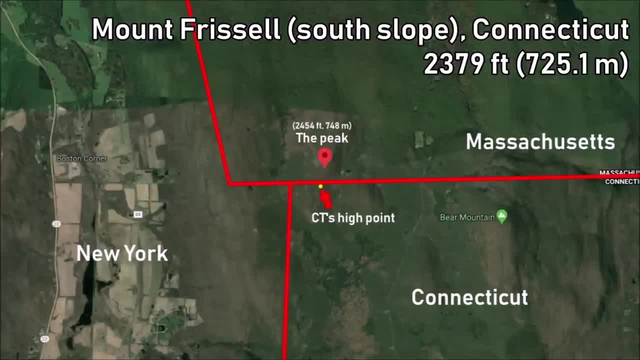 In Connecticut, the high point is at 2,379 feet and is located about 1,000 feet away from the tri-points of Connecticut, Massachusetts and New York. In Alabama, Cheehaw Mountain at 2,413 feet is the highest point in the state. 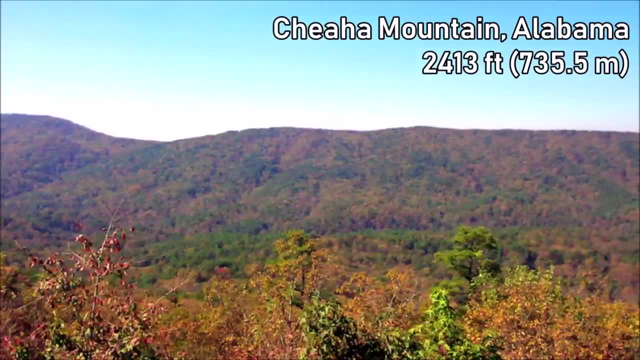 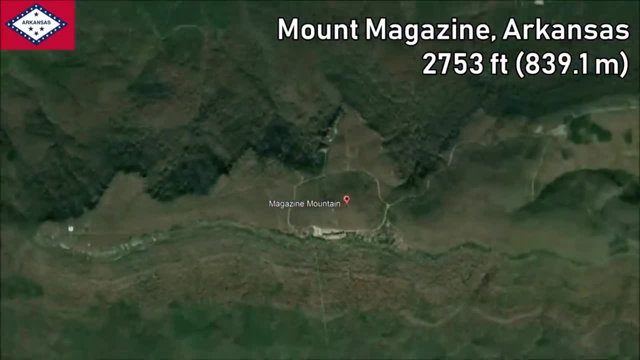 It's part of the Talladega mountain range and appears to be much higher than it is due to its prominence. Arkansas- perhaps the first state of the video so far- that's well-known for having mountains, has its highest point at the 2,753-foot peak of Mount Magazine. Although it's very close to the Ouachita Mountains, it's technically a formation of the Arkansas River Valley instead and is part of the Ozark National Forest. Similarly to Arkansas's mountainous fame, Pennsylvania is famous for the Appalachian Mountains, which are home to its high points of Mount Davis, located near the border with Maryland. Mount Davis comes in at 3,213 feet. Speaking of Maryland, its high point of Hoy Crest is next in line, At an elevation of 3,360 feet. it's found just barely across the border with West Virginia and is part of the Backbone Mountain Ridge. I mentioned Massachusetts a while back and it makes its appearance now with Mount Greylock. Its elevation of 3,489 feet and location in the northwest corner of the state provides beautiful views of five states and is also home to the only taiga forest in the state. There's also a paved road to the top and a war memorial tower at the summit. North Dakota brings us the first high point of the American West, with White Butte At 3,506 feet. it's set among the Badlands of Western North Dakota and is on private property. 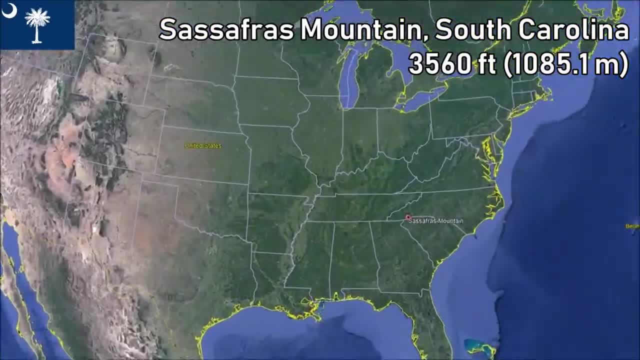 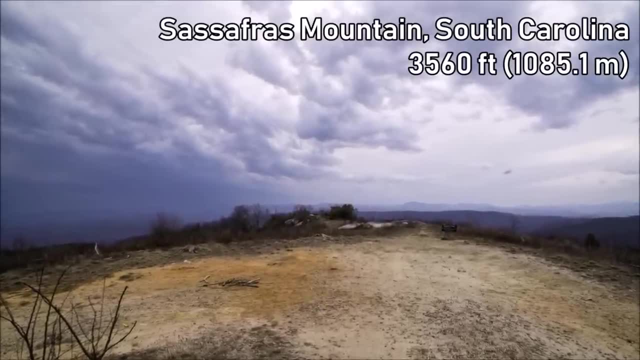 South Carolina takes us back to the Appalachians. Its highest point, Sassafras Mountain, is split in two by the border with North Carolina in the Blue Ridge Mountains and is at an elevation of 3,560 feet To reach the observation tower, which is on the South Carolina side. 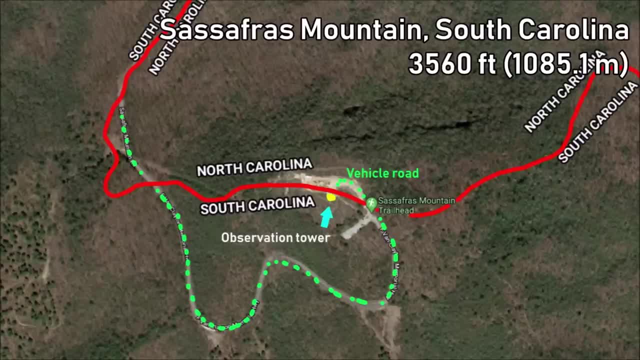 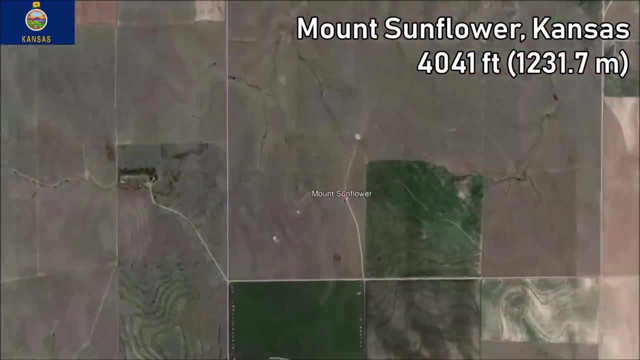 visitors have to pass through North Carolina first, if they stay on the path. In Kansas we find Mount Sunflower, one of the more famous high points of the 50 states. It's not an actual mountain or hill or really anything. 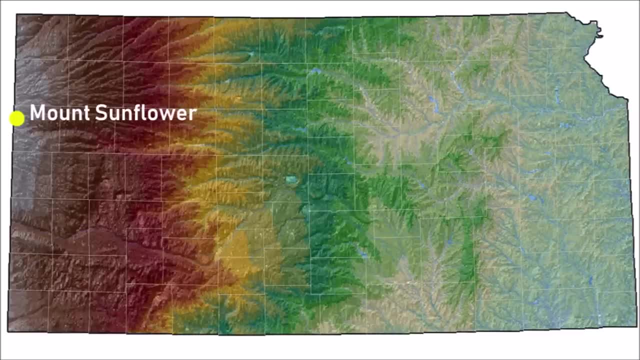 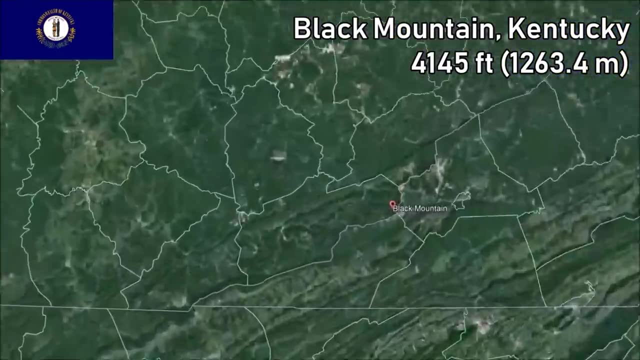 but just the end of the long gradient of elevation that is the state of Kansas. about half a mile from the Colorado border, Kentucky has an actual mountain, a mountainous high point, of course, being Black Mountain. It's just over the border from Virginia, in the eastern part of the state. 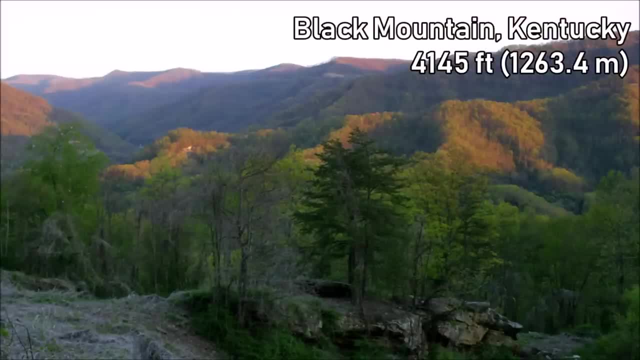 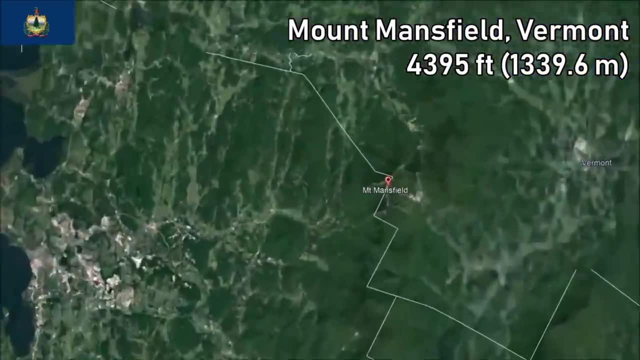 and is easily accessible by road. It comes in at 4,145 feet. Vermont, the Green Mountain state, has Mount Mansfield to claim as its high point, at an elevation of 4,395 feet, While the summit is a destination for high-pointers. 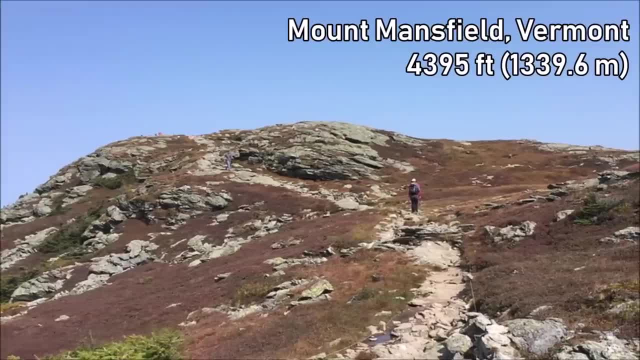 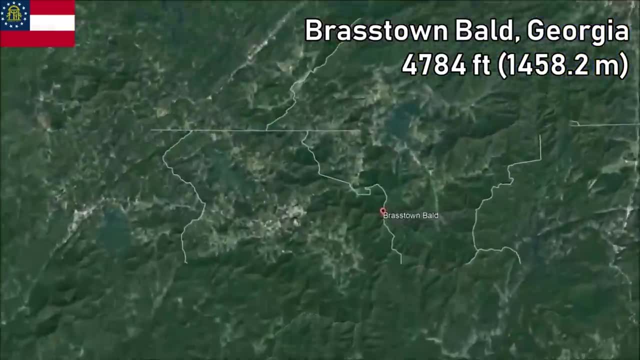 the mountain is also a ski resort and features some of Vermont's last remaining alpine tundra from the Ice Ages. Back south to Georgia we find Brasstown Bald, a 4,784-foot-high mountain peak found in the Chattahoochee National Forest of northern Georgia. 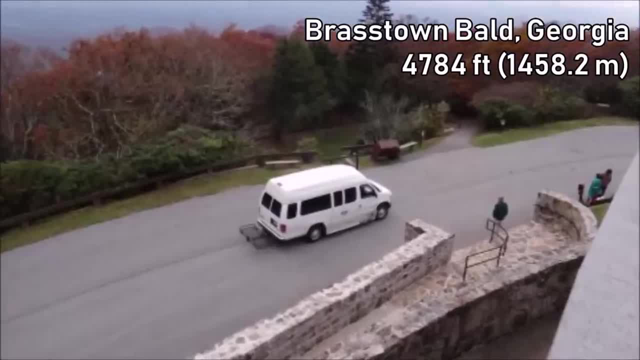 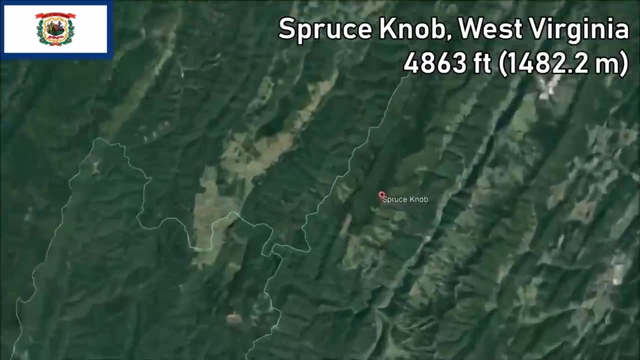 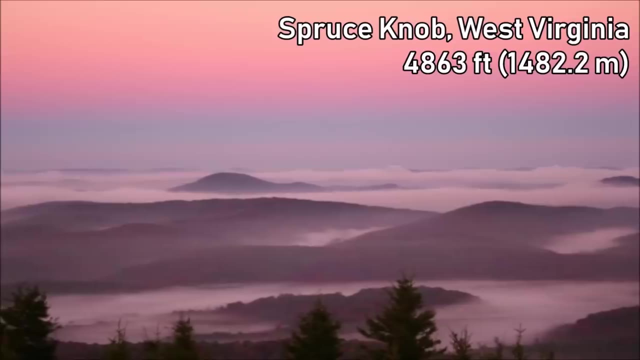 There's apparently a shuttle service that runs to the top very frequently. How convenient, Ah, West Virginia, an almost heavenly state, famous for its Blue Ridge Mountains and Shenandoah River. Its country roads will take you to the place you belong. Spruce Knob, its highest point at 4,863 feet. 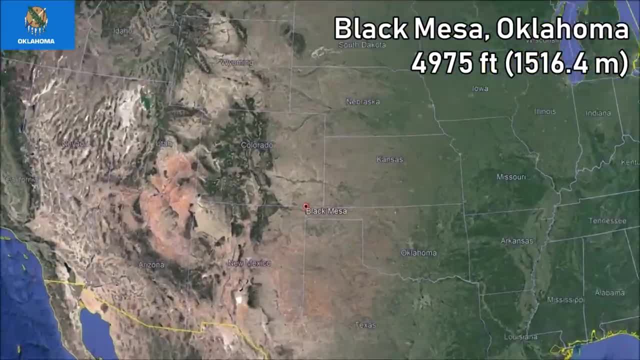 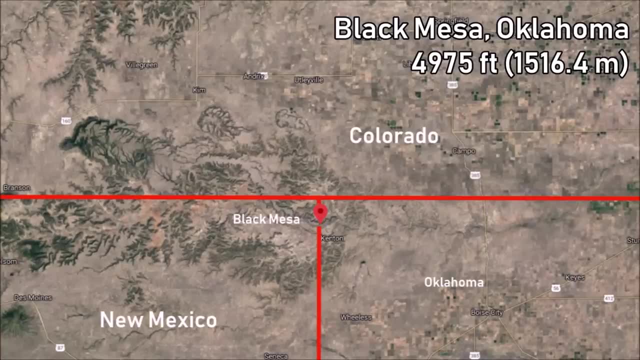 found just outside the eastern panhandle In Oklahoma. the highest point is found on Black Mesa, a mesa which just barely stretches into the panhandle, coming out of New Mexico At 4,975 feet, the area is a quite different landscape from what most people think of when they hear Oklahoma. 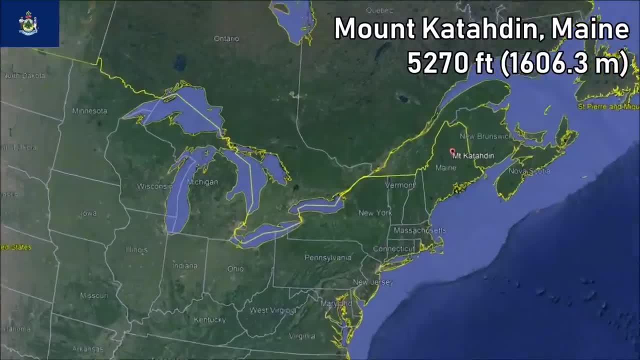 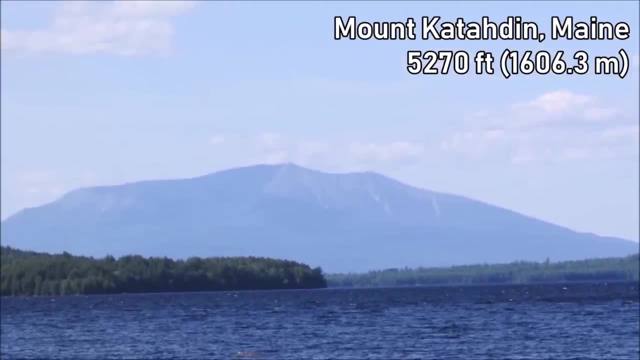 It is a beautiful spot, though. Up in Maine there's Mount Katahdin at an elevation of 5,270 feet. This mountain is found quite centrally in the state of Maine and is also noteworthy as the northern end of the Appalachian Trail. 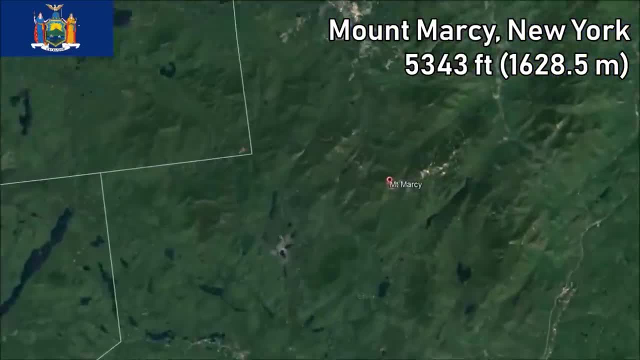 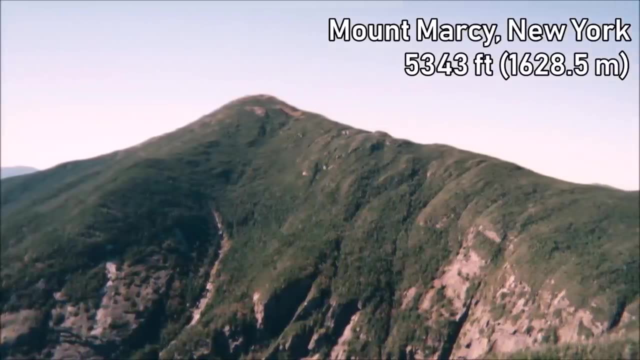 Close by New York has Mount Marcy, found in the northern part of the state among the Adirondack High Peaks region. With an elevation of 5,343 feet and not being too far away from Lake Placid, it's a very popular destination in the area. 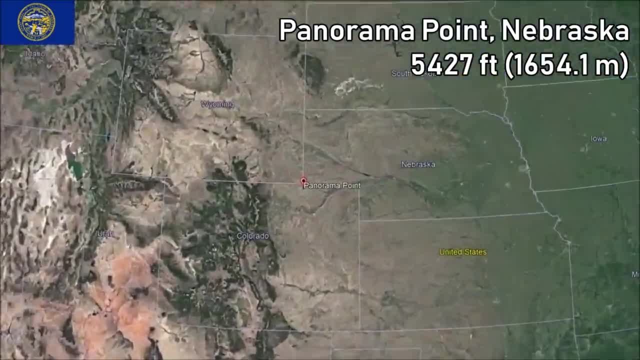 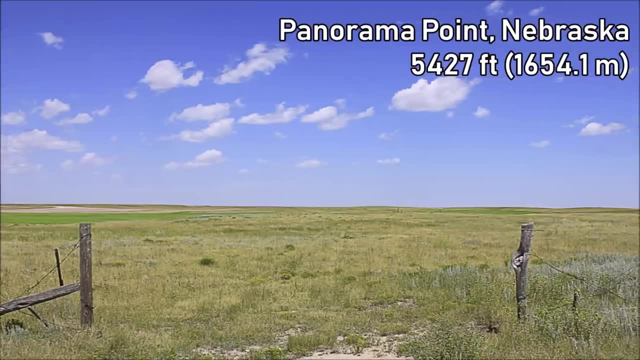 and offers great views Back in the Plains. Nebraska's high point is Panorama Point at 5,427 feet Quite. similarly to neighboring Kansas, Panorama Point has very little noticeable prominence and is found just over the border from Colorado and Wyoming. About a mile away from the tri-point of the three states. Virginia also has a high point that's not too far from a tri-point. Mount Rogers, at 5,729 feet, is evidence of former volcanic activity in the Appalachians hundreds of millions of years ago. It's in far south Virginia, near the tri-point with Tennessee and North Carolina. New Hampshire brings us another famous high point, Mount Washington, Coming in at 6,288 feet. it's found in the northern half of the state and is well known for its extreme winds. 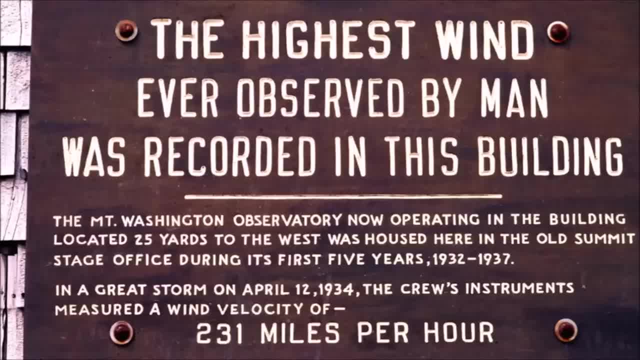 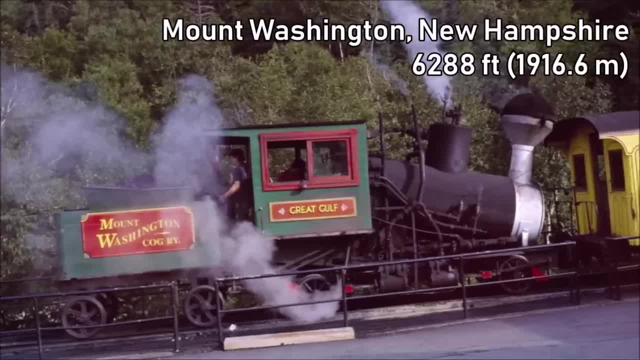 The fastest wind speed ever recorded. that wasn't found in a tornado or hurricane: 231 miles per hour was measured at the summit. That's insane. There's also a cog railroad and a vehicle road that climbs to the top. Tennessee is home to Clingmans Dome. 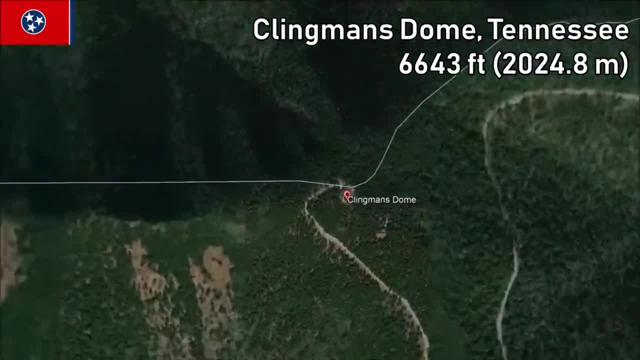 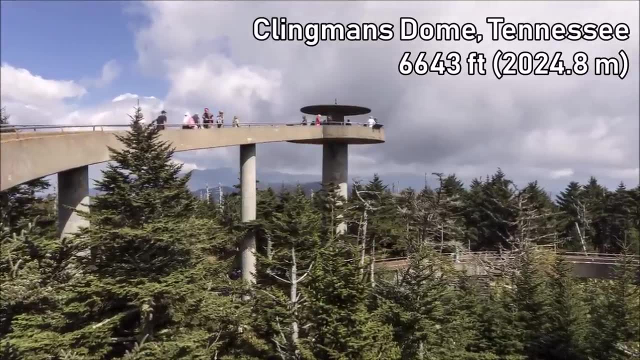 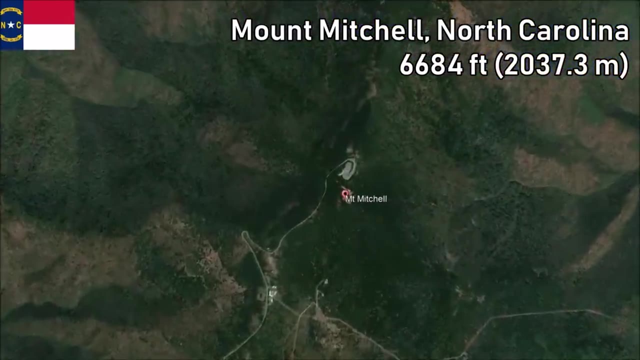 a mountain shared with North Carolina in the Great Smoky Mountains. Atop the 6,643 foot summit is an observation deck and the entire area is accessible by car. Not far away at all, North Carolina's Mount Mitchell lays claim to the highest point in the state, at 6,684 feet. 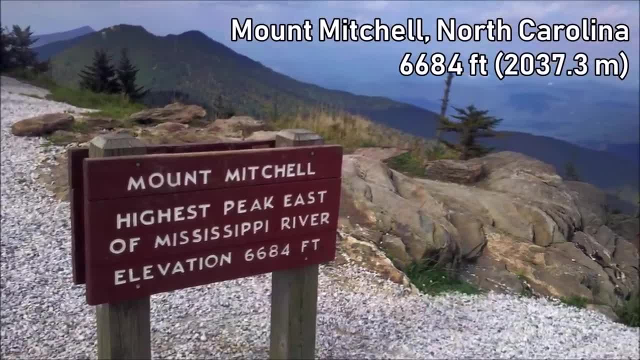 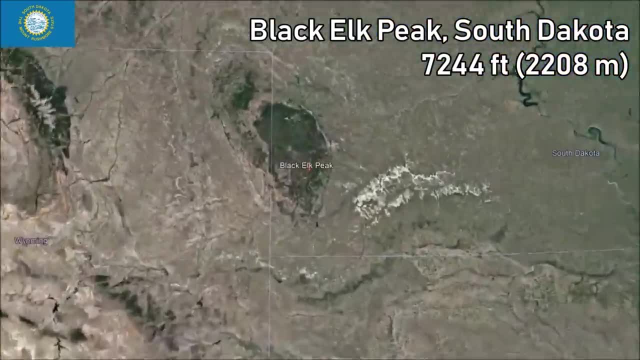 It's also the highest point found east of the Mississippi River and is quite the popular destination. as a result, From here on out, we'll be dealing with exclusively western states. Starting us off is South Dakota, with its 7,244 foot Black Elk Peak. 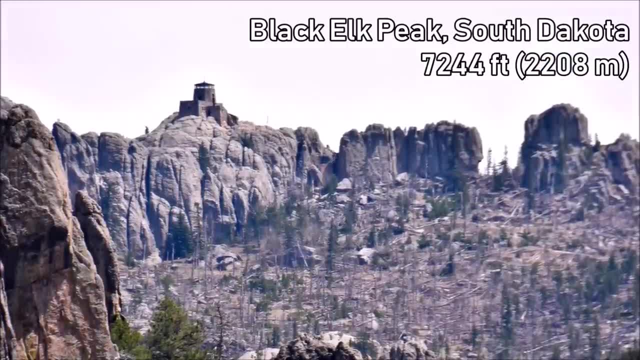 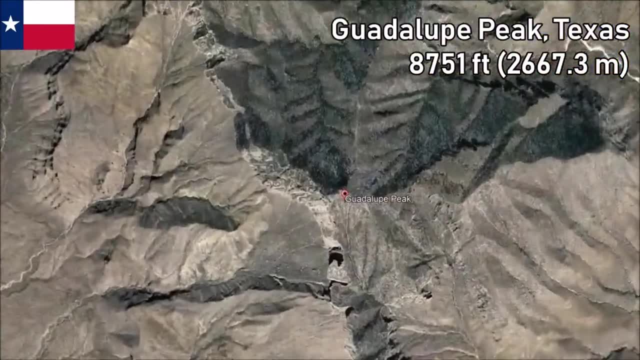 found in the Black Hills just a few miles away from Mount Rushmore, Texas makes its appearance with Guadalupe Peak, found in West Texas in the Guadalupe Mountain Range shared with New Mexico At 8,751 feet. 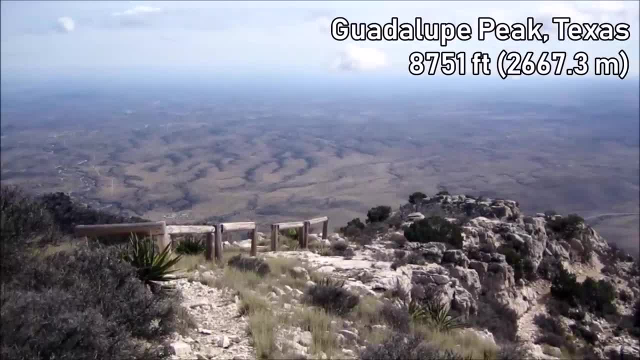 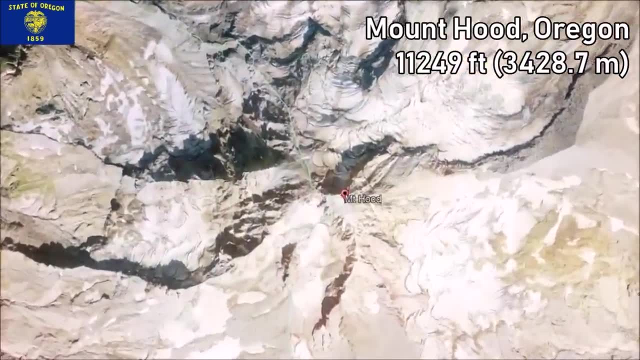 there is a hiking trail all the way to the top, with great views of the surrounding desert. Oregon's highest point is Mount Hood, a quite well known peak towering nearby to Portland, and the first peak over 10,000 feet on the list. 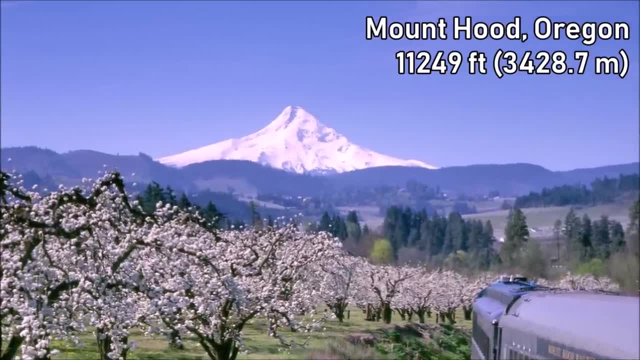 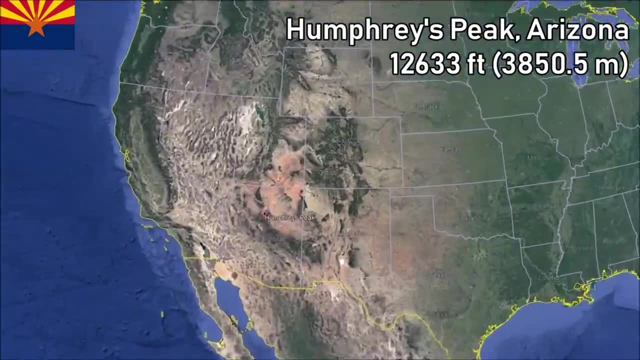 coming in at 11,249 feet. It's also part of the Cascade Volcanic Arc and is a potentially active volcano itself. Arizona has Humphreys Peak as its highest point, just north of Flagstaff in the San Francisco Peaks. 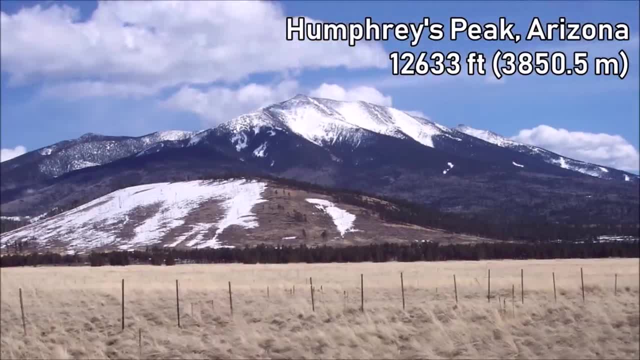 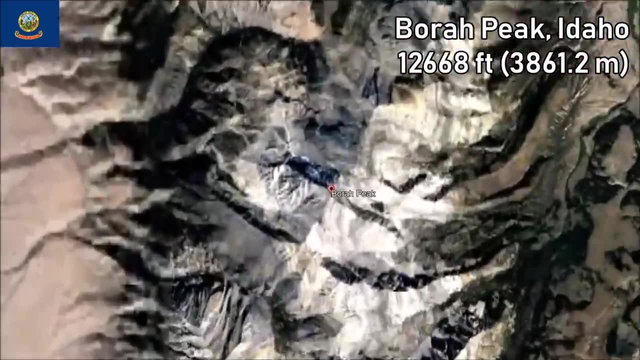 It has an elevation of 12,633 feet and offers great views of the surrounding area. Idaho's highest point is Bora Peak, situated in the center of the state among the Lost River Range. Its elevation is 12,668 feet. 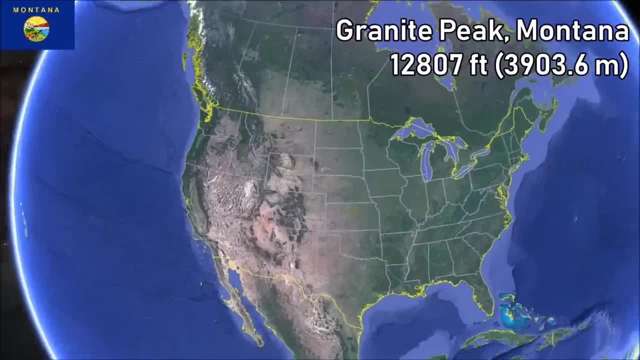 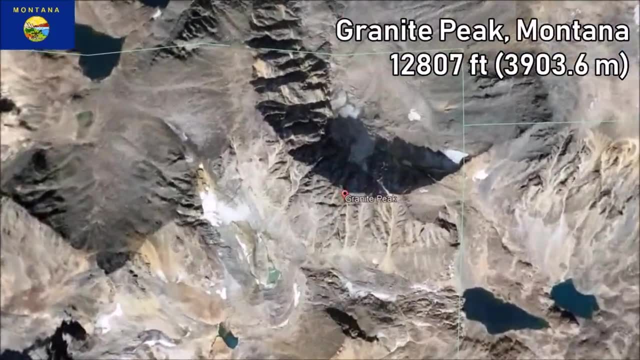 and features quite a strenuous hike to the summit. Up in neighboring Montana is Granite Peak found 10 miles north of the border with Wyoming. At 12,807 feet, it's widely regarded as the second most difficult high point to ascend. 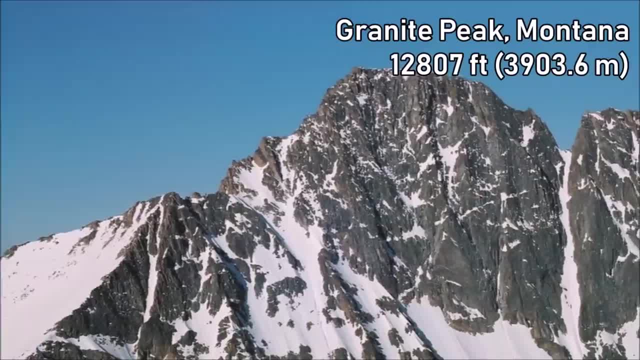 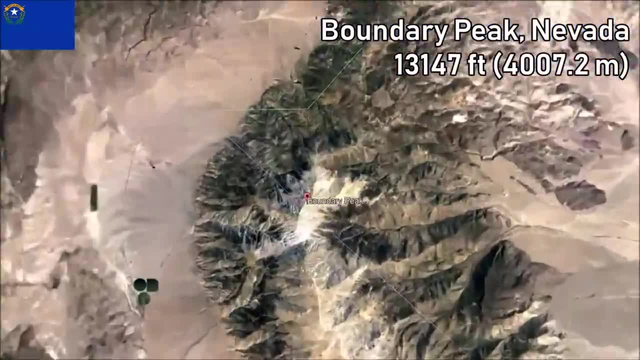 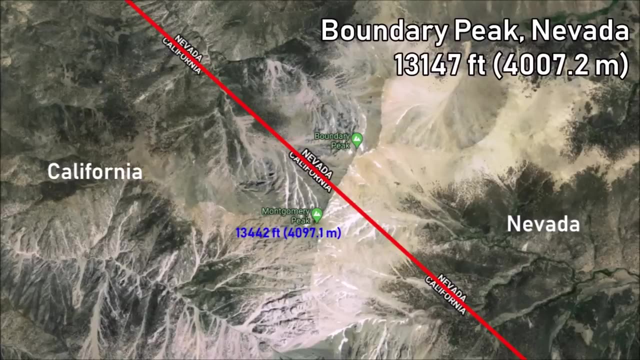 due to its weather conditions- tricky, routing, and it usually takes at least two days to climb. Nevada's highest point is the 13,147 foot high Boundary Peak, aptly named, as it lies just over the border with California. It's technically a sub-peak of California's taller Montgomery Peak. New Mexico's highest point is just barely taller, at 13,167 feet, found at the summit of Wheeler Peak. The area is very close to Taos and skiing and hiking are popular activities. Over in Utah is Kings Peak, at an elevation of 13,534 feet. 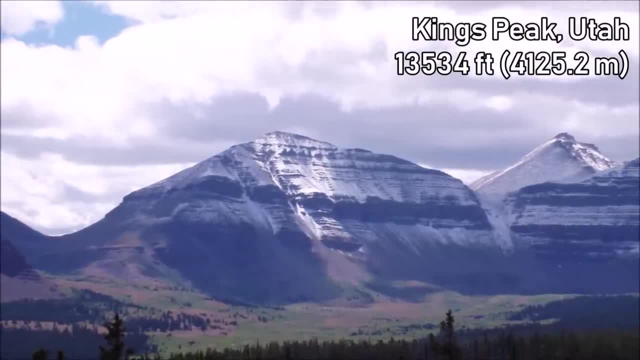 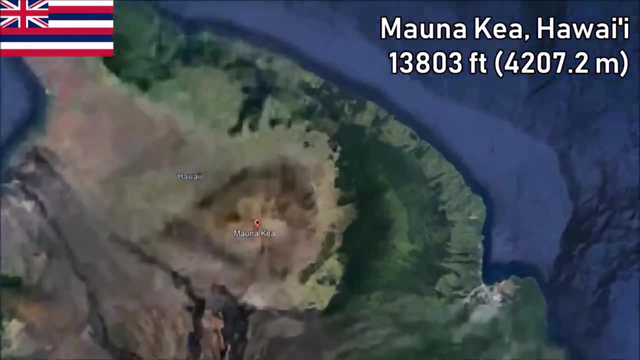 It's found in the Uinta Mountains of northeastern Utah, not too far away from the Wyoming border. We're venturing away from the lower 48 for the first time, with Hawaii's famous high point of Mauna Kea At 13,803 feet above sea level. it's sometimes considered to be the tallest mountain in the world when measured from its true base at the seafloor. It's home to many astronomical observatories, is held sacred by native Hawaiians and is famous around the world, Starting out the top five of this list. is Wyoming's Gannett Peak at an elevation of 13,809 feet. It straddles the Continental Divide and is part of the Wind River Range. Next up is Washington's world-famous Mount Rainier, the 14,411 foot high active volcano. 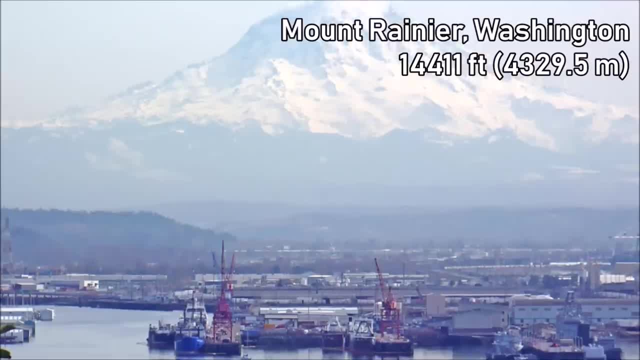 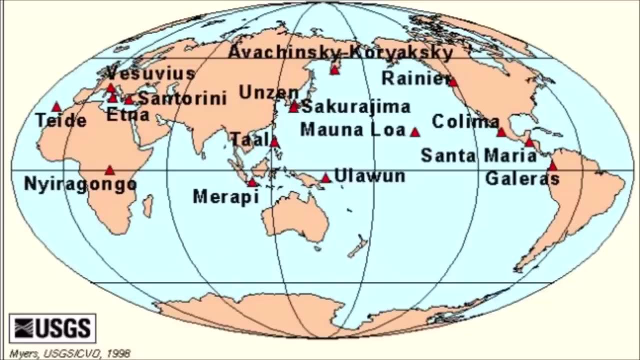 looming in the distance near the Seattle region. It's considered to be one of the most dangerous volcanoes in the world and is a decade volcano, one of 16 volcanoes designated as the most important to study. Third place goes to Colorado's Mount Elbert. 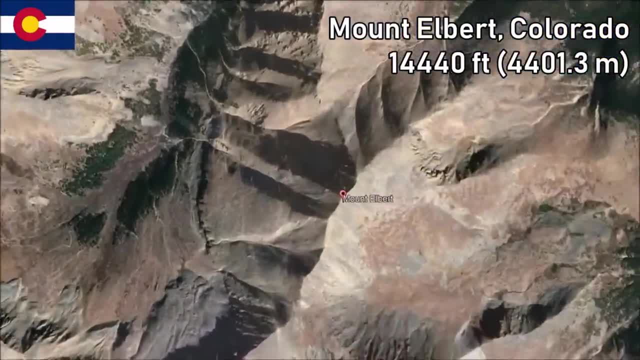 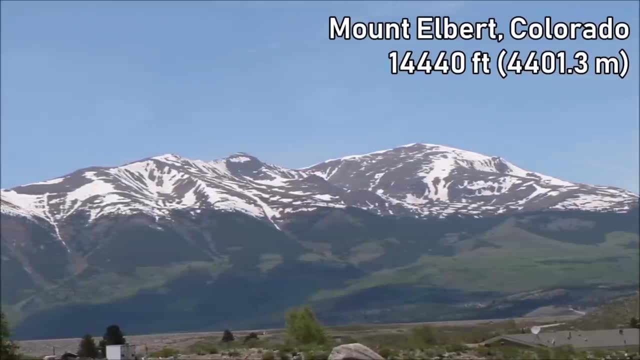 which is featured in this video's thumbnail. It comes in at an elevation of 14,440 feet. It's the highest point of the entire Rocky Mountain Range. Considering its high elevation, it's not a particularly difficult peak to ascend, relatively. 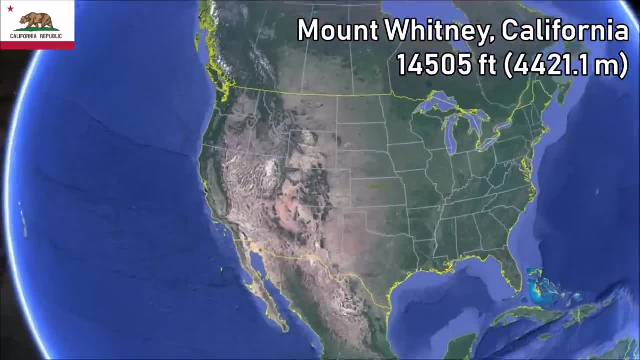 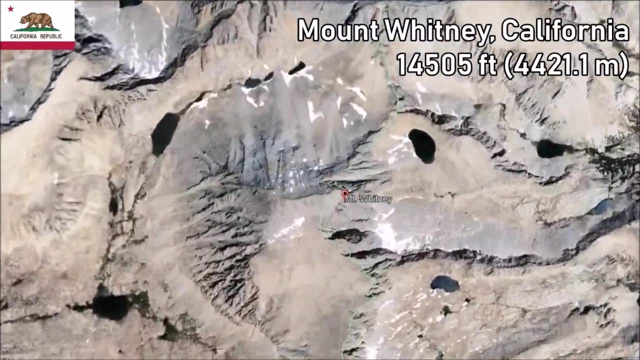 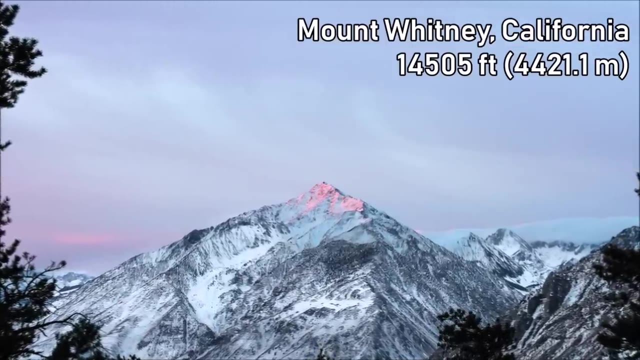 which earned it the nickname of the Gentle Giant. California and its Mount Whitney claim the second highest state high point, with an elevation of 14,505 feet. It's also the tallest mountain of the entire lower 48 states, which leaves just one more state left to claim first place. 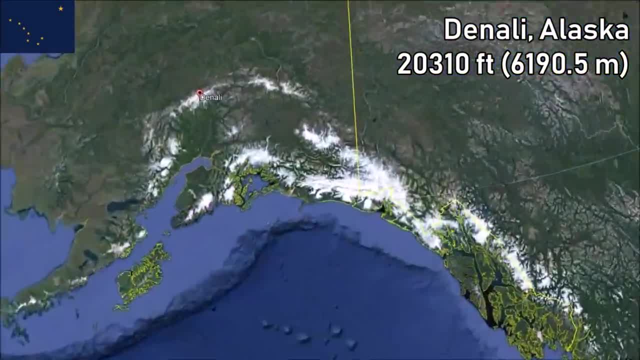 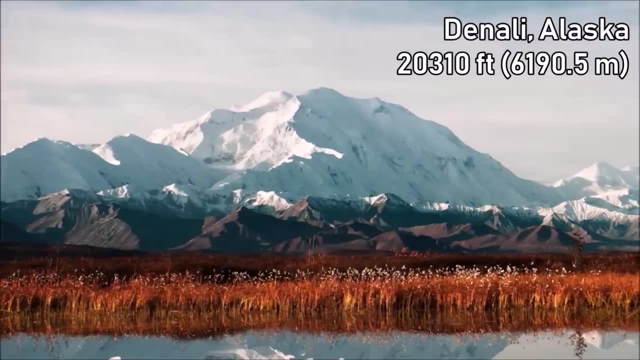 Alaska and its famous Denali take the spot of the highest high point of all 50 states, with an astounding elevation of 20,310 feet. It was known as Mount McKinley until 2015.. It's the third most prominent mountain on Earth. 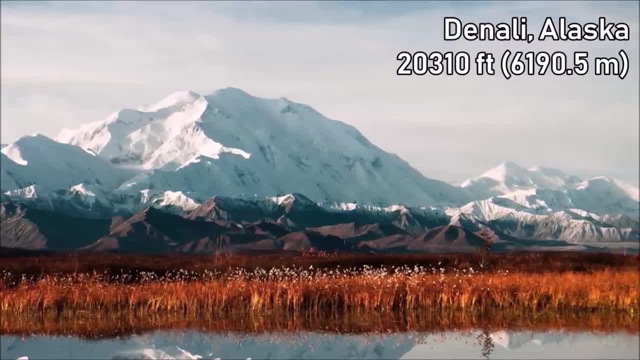 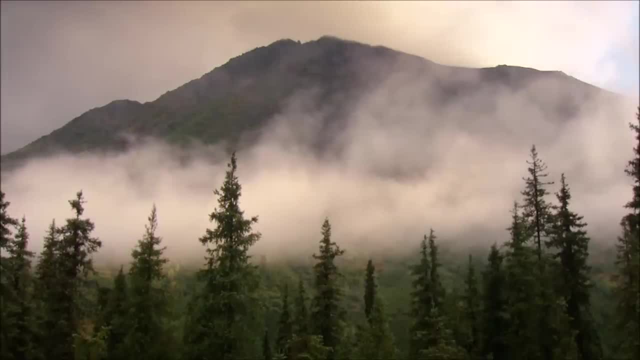 and the tallest peak in North America. What an impressive place. And that concludes this. look at every state's high point. From vacant lots in the suburbs to towering peaks in the remote wilderness, the USA truly does offer an incredible variety of high points. 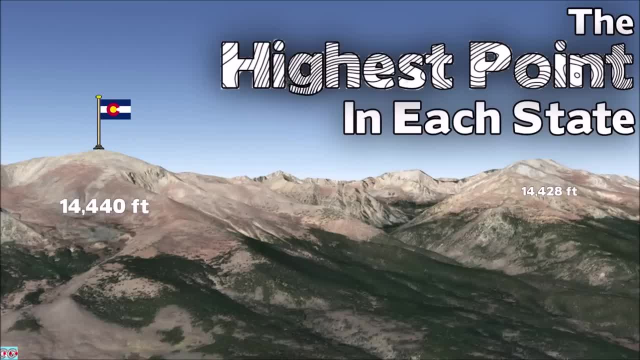 Thank you for watching the video all the way through. If you enjoyed it, I'd greatly appreciate it if you checked out some of my other similar videos and subscribed. Have a great day and I'll see you next time. 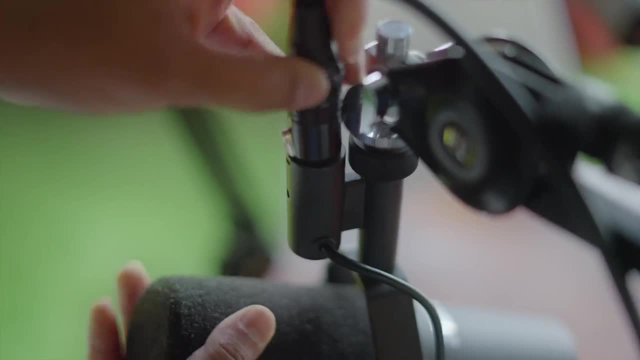 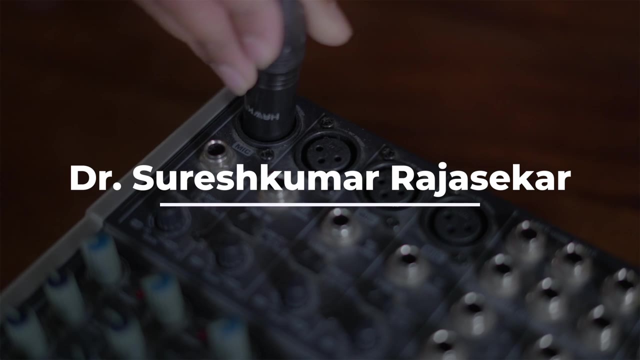 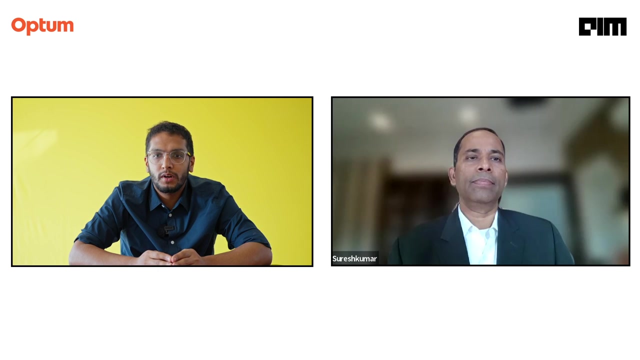 Hello and welcome everyone to the next episode of the Analytics India Magazine podcast, Simulated Reality. Today we have with us Suresh Kumar Rajasekhar. He is the VP of Technology at Optum Global Solutions. Welcome, Suresh, how are you today? 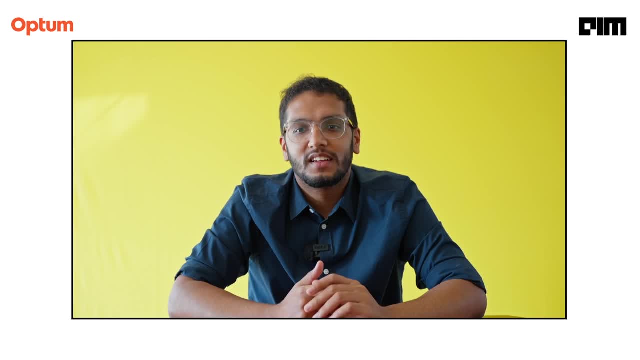 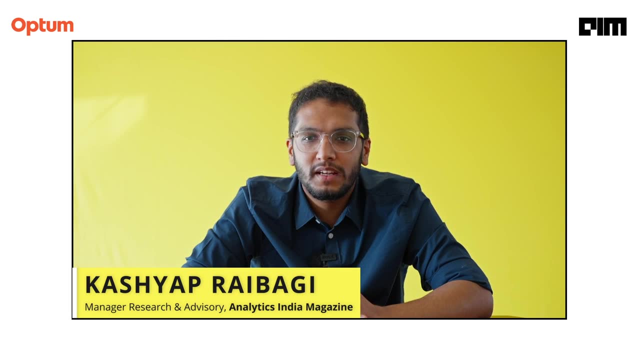 Hey, doing great. Kashyap, Nice meeting you. Yes, likewise. So I think we are going to speak a very topic that has been discussed heavily, especially after the COVID-19 pandemic, and that is the use of data, data analytics, data science. 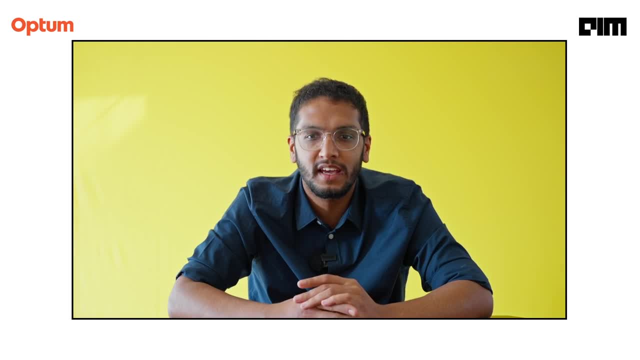 AI and all these emerging technologies in the field of healthcare. But I just want to take a step back and before we kind of understand why we use data, most leaders, technology leaders such as yourself- say that first you have to understand the problems. You don't. 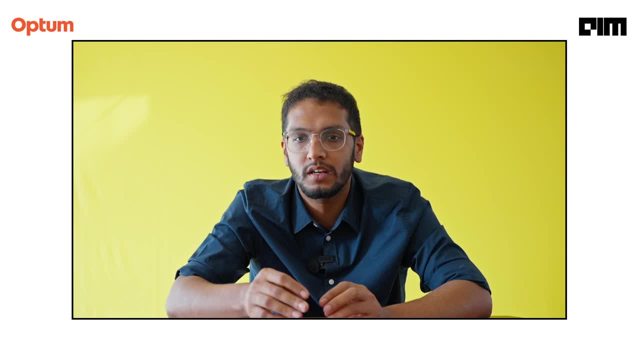 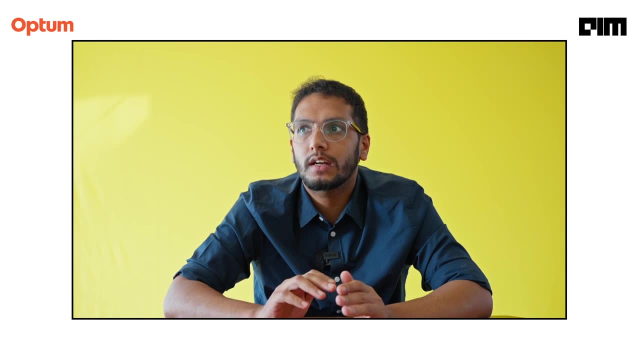 start with the data and say that let me take data and solve it with it. What are some of the problems that have existed? Because healthcare as a field, we have collected a lot of data. It may be not- and the entire digitization process we can discuss later, but it has always collected a lot. 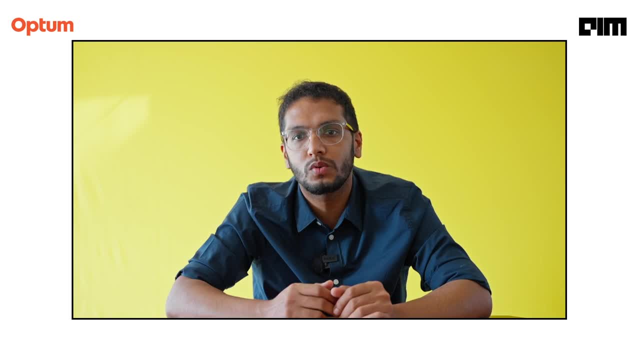 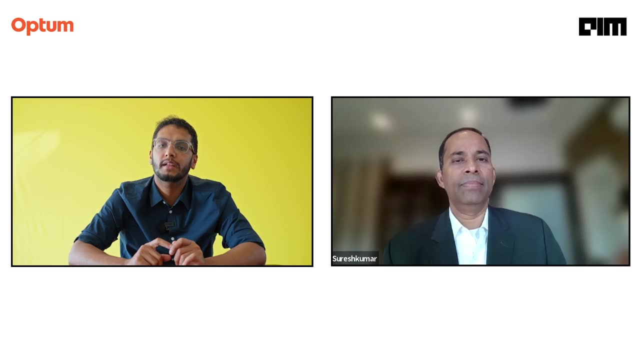 of data? What has historically, and then maybe closer to 2022, as we enter 2023, what have been some of the problems in healthcare that data analytics have been identified to be the best solution, And why do you think data is the best solution for them? Thanks for asking that. 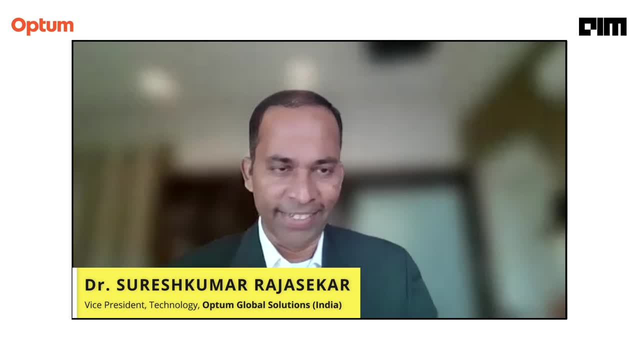 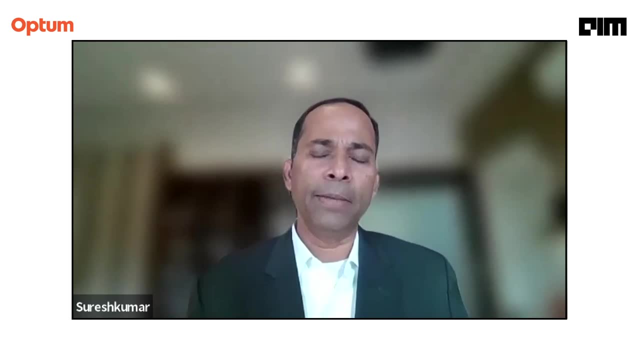 you know like, instead of directly jumping into where we can apply cookie cutter right? Thank you, Yeah, I think I understand. you know, first of all, the healthcare landscape a little bit. Institute of Health Improvement- IHI. almost 15 years back in 2007,, they identified patient.